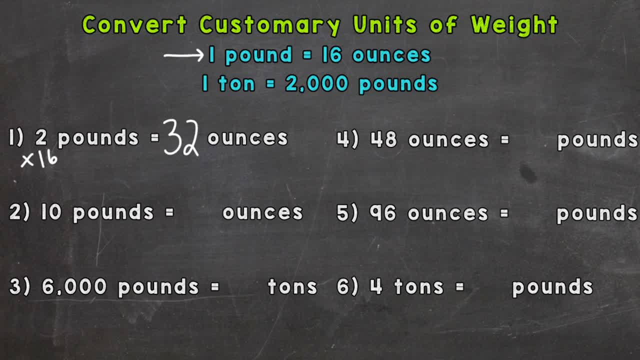 equals how many ounces. So 16 plus 16 plus 16, 10 times 10 groups of 16.. So we can do 10 times 16 to solve this, And 10 times 16 equals how many ounces. So we have: 10 pounds equals how many ounces. 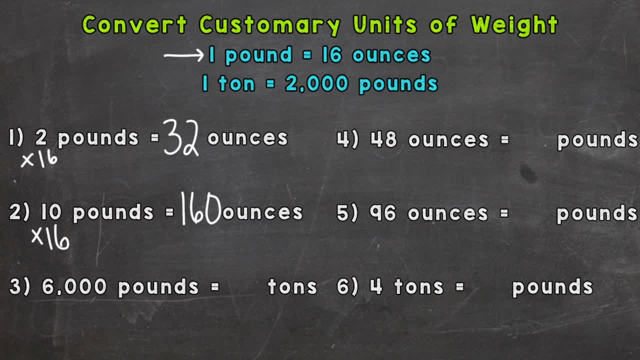 So 10 pounds equals 160.. So 10 pounds equals 160 ounces. Now for number three. we're going to go pounds to tons, So 6,000 pounds. Well, we know one ton equals 2,000 pounds, So we need to find. 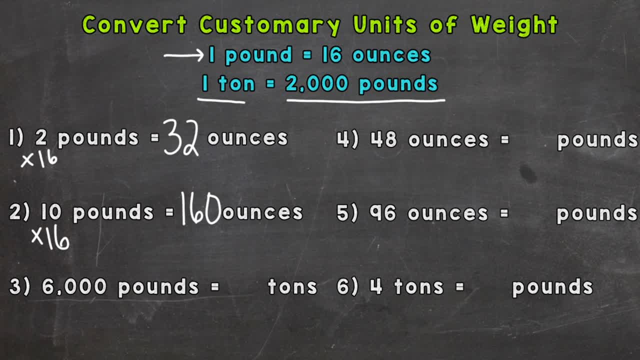 how many groups of 2,000 can we pull out of 6,000.. Because each of those groups of 2,000 is a ton. So we need to find how many groups of 2,000 can we pull out of 6,000.. So we need to. 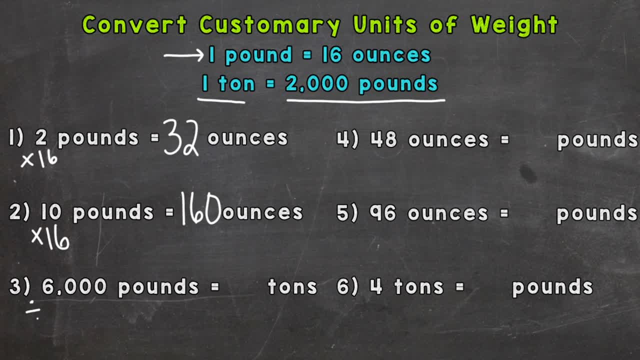 do 6,000 divided by 2,000.. And that's going to give us 3.. So the 2,000 is one ton plus another 2,000 is two tons, plus that last 2,000 is three tons. Number four, 48 ounces, equals how many? 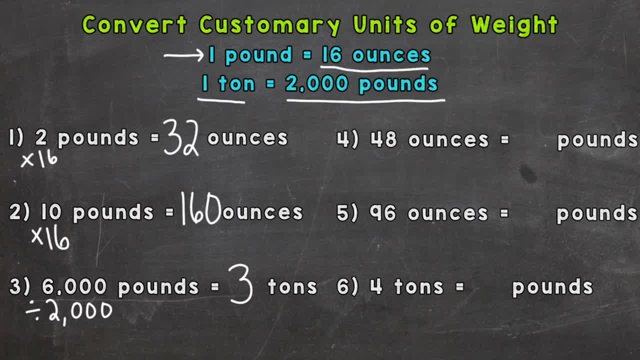 pounds. Well, we know 16 ounces equals one pound. So we have: 10 pounds equals 16 ounces. So we need are going to have to split that 48 ounces into groups of 16. And each of that group, each of those groups of 16, equals one pound. So let's do 48 divided by 16. And 48 divided by 16 is three. 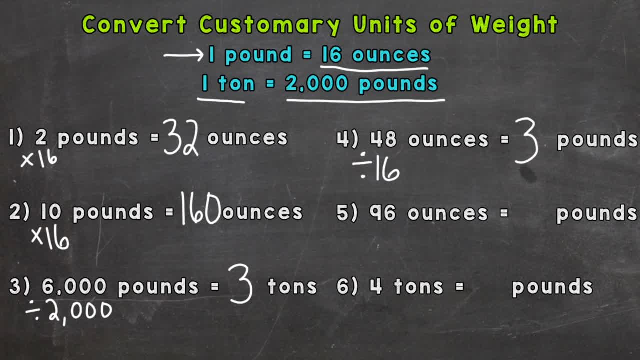